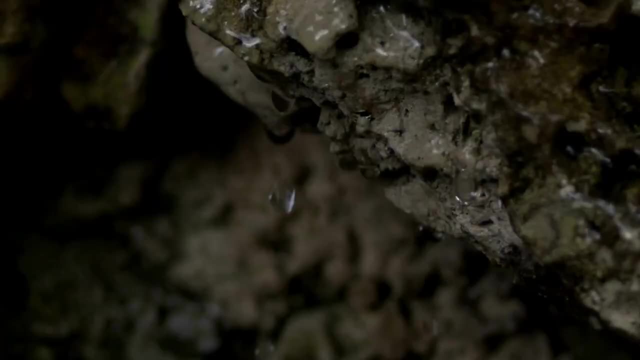 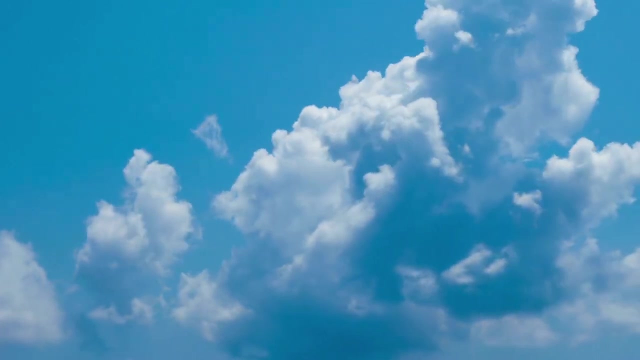 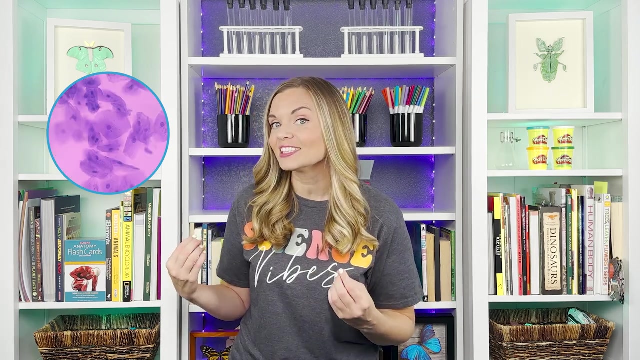 water dripping down into underground aquifers, and even water as vapor floating around just waiting to mix with dust to become clouds. Water is hanging out in plants and animals and even in the very cells that make up us. The biosphere contains all living organisms on Earth, from giant blue whales to the tiniest bacteria. 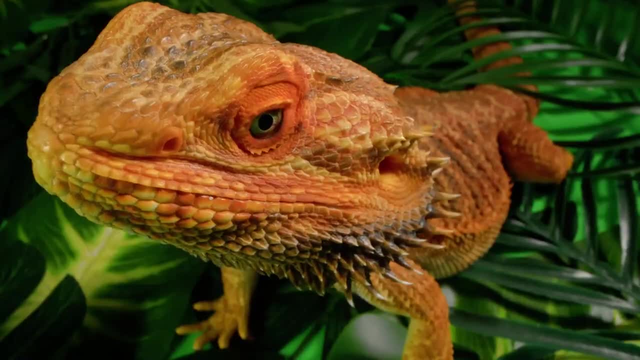 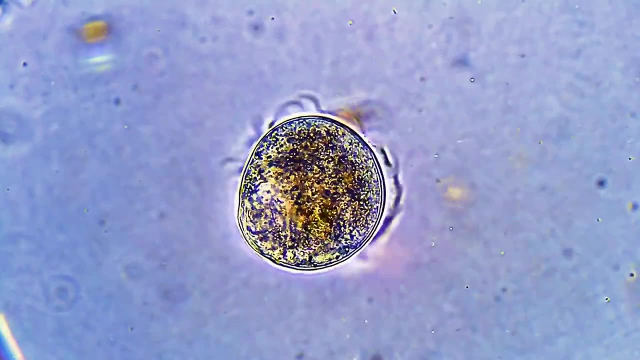 reptiles, insects, arachnids, birds and even humans, And that's it, That's it. That's it. Mammals, plants, fungi and even tiny organisms. you need a microscope to see If it's living. it belongs to this sphere. 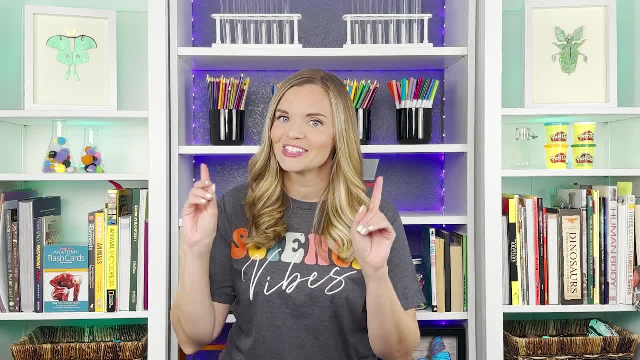 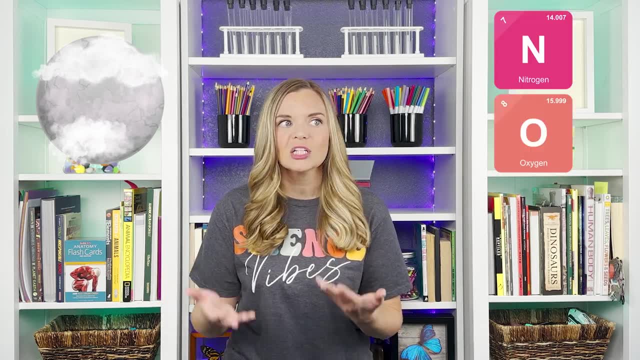 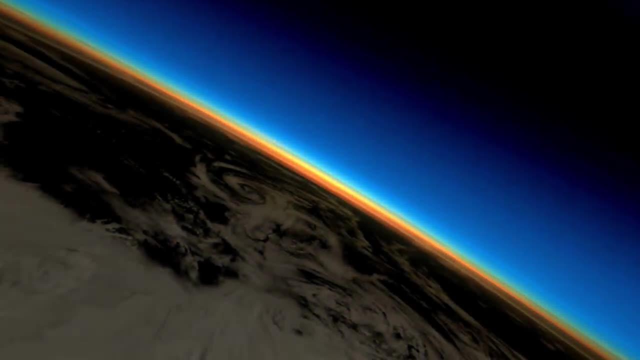 If you're not sure exactly what is living, you can check out this video. The atmosphere contains all the gases floating around us, Gases like nitrogen, oxygen, argon and carbon dioxide, to name a few. You can think of the atmosphere like this nice protective blanket for our planet. 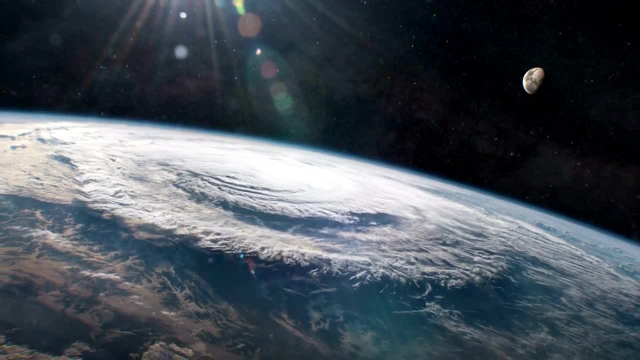 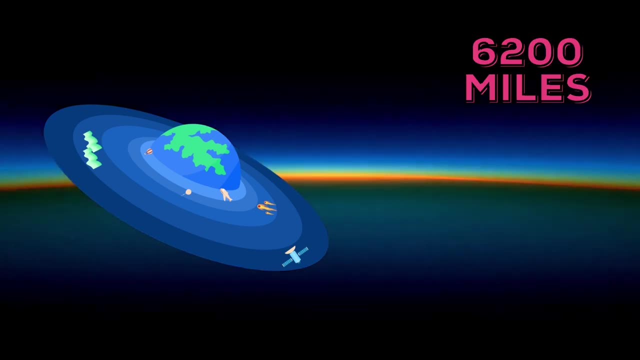 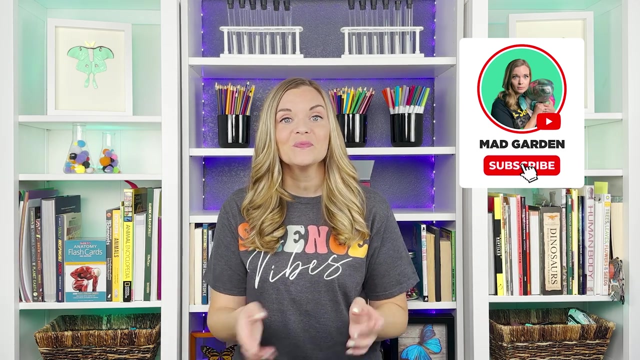 It protects us from things like Radiation from the Sun And breaks up small space rocks that might bump into our planet. The atmosphere extends about 6200 miles above Earth's surface and contains several layers. If you're still here liking this video, hit that subscribe button so you never miss an episode. 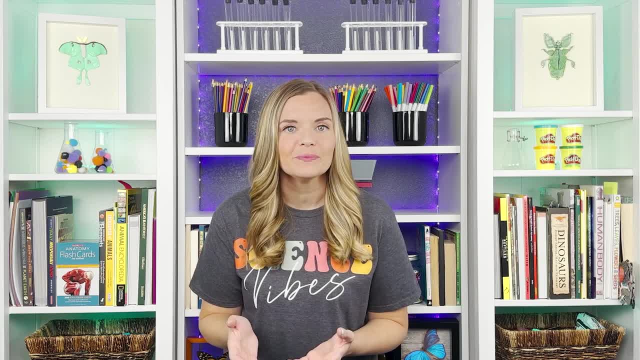 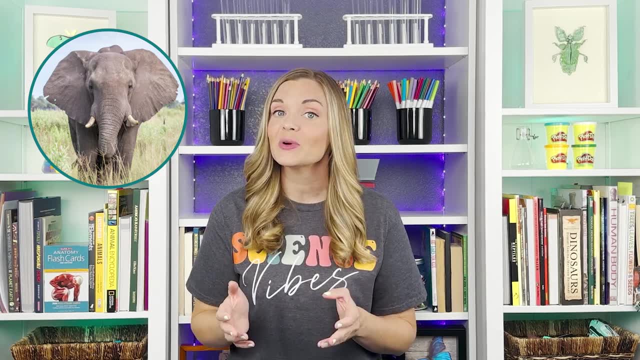 Like we learned earlier, these spheres aren't separate. they're constantly interacting with each other. Let's take a look at an elephant to see how this living organism interacts with each sphere. These elephants are stopping at a pond for a drink. This pond belongs in the 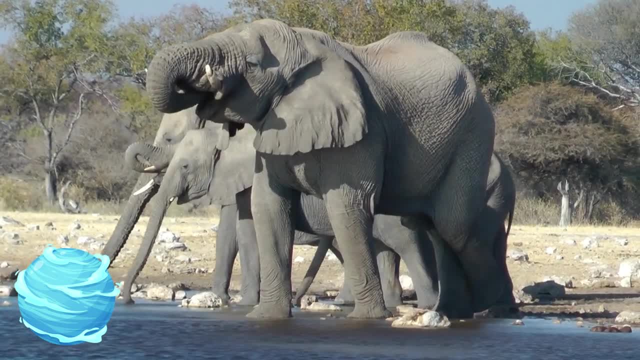 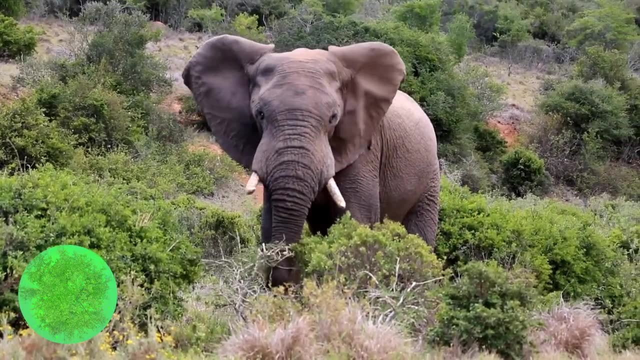 hydrosphere and that water is going to travel through the elephant's body and even become part of its cells. This elephant is eating lunch. This plant belongs to the biosphere, as does the elephant. These guys are having a dust bath, This coating of dirt on their skin. 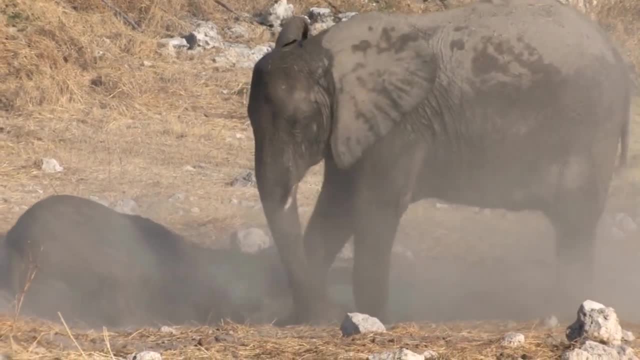 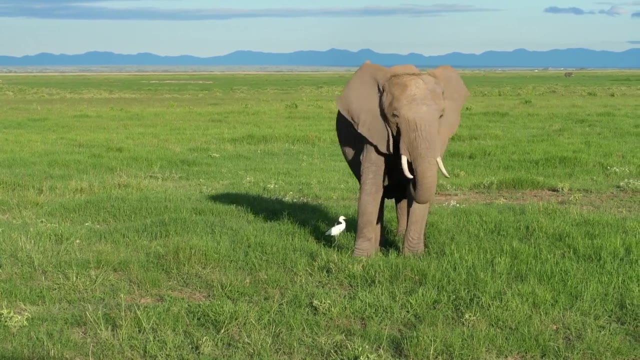 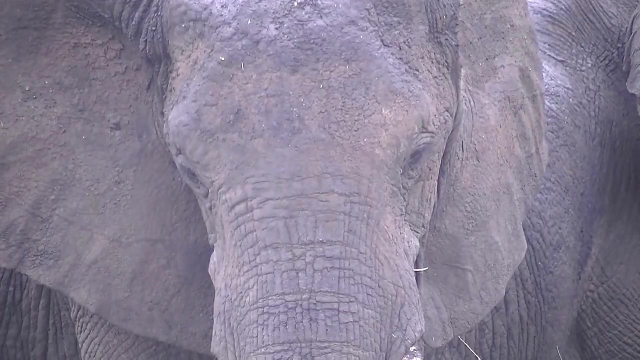 provides UV and pest protection. The dirt belongs to the geosphere. This elephant and the white cattle egret here have a symbiotic relationship. As the elephant feeds on the grass, small insects are kicked up and become a nice snack for the bird. This guy is getting rained.